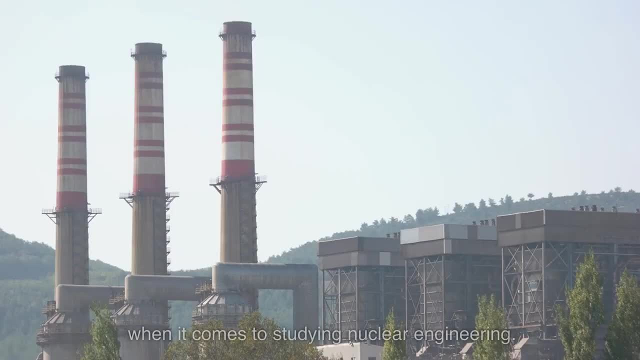 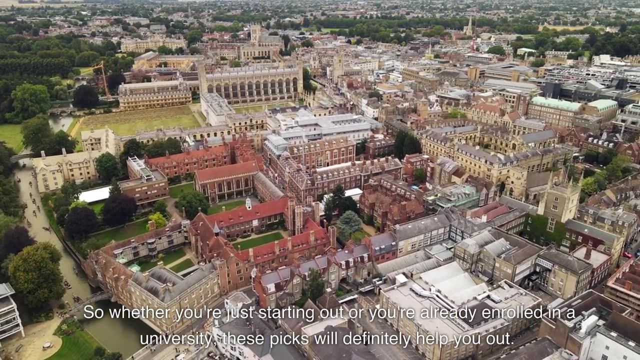 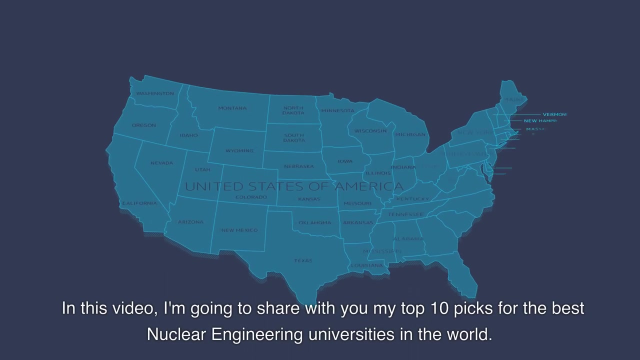 Top Nuclear Engineering Universities in the World When it comes to studying nuclear engineering. So whether you're just starting out or you're already enrolled in a university, these picks will definitely help you out. Hello and welcome to my channel, Top USA Entertainment. In this video, I'm going to share with you my top 10 picks for the best nuclear engineering. 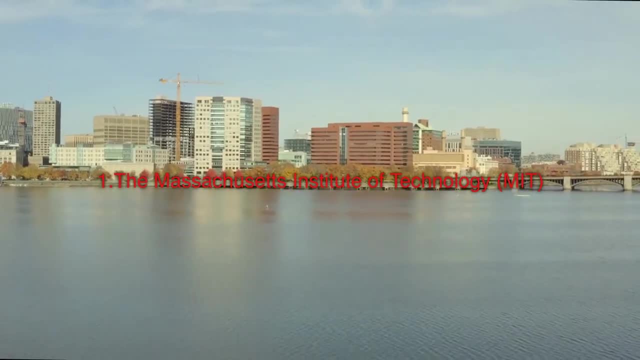 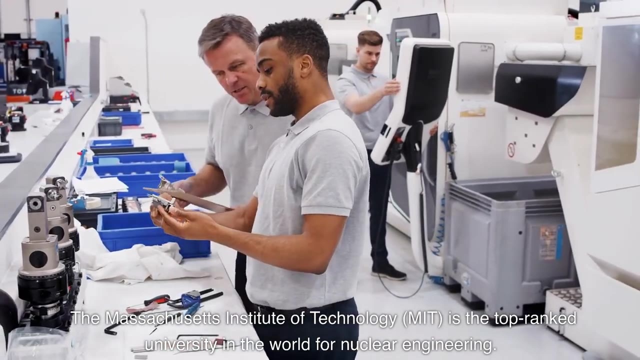 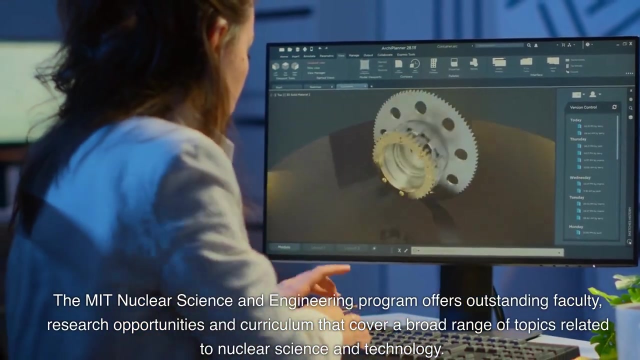 universities in the world. 1. The Massachusetts Institute of Technology. The Massachusetts Institute of Technology is the top-ranked university in the world for nuclear engineering. The MIT Nuclear Science and Engineering program offers outstanding faculty research opportunities and curriculum that cover a broad range of topics related to nuclear science. 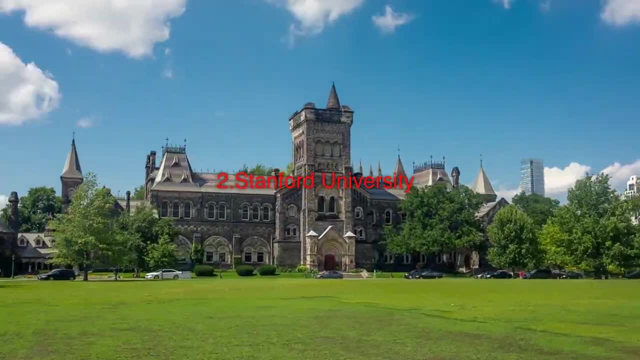 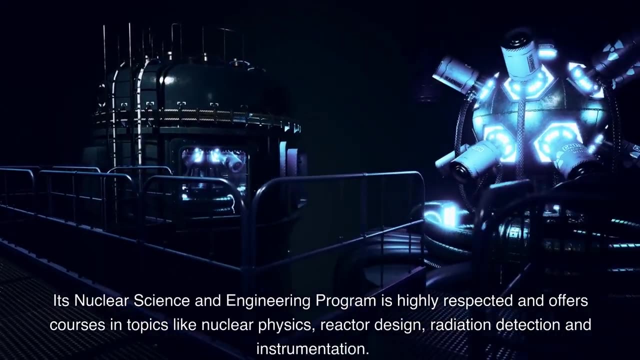 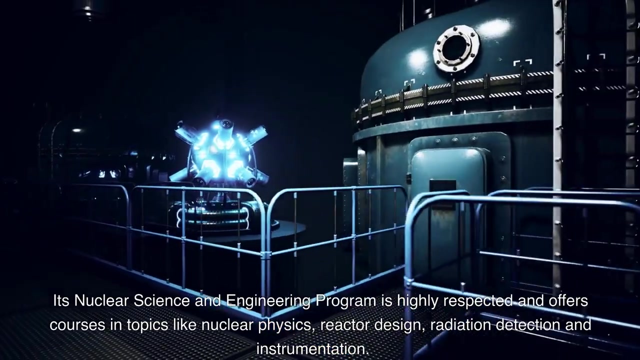 and technology. 2. Stanford University. Stanford University is another top choice for nuclear engineering students from around the globe. Its Nuclear Science and Engineering program is highly respected and offers courses in topics like nuclear physics, reactor design, radiation detection and instrumentation. 3. University of California, Berkeley. 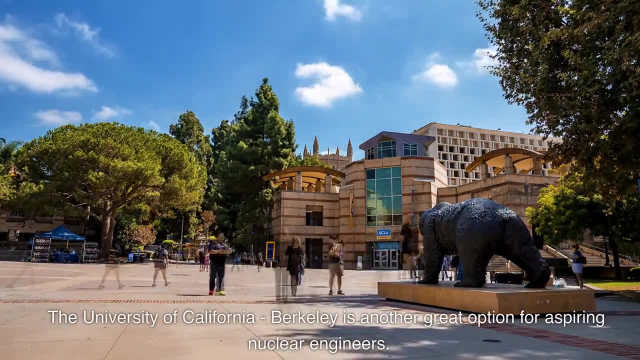 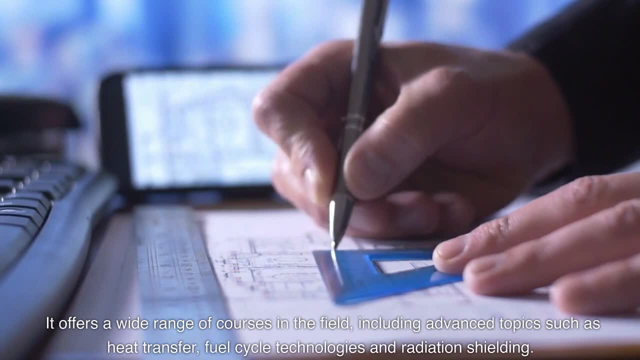 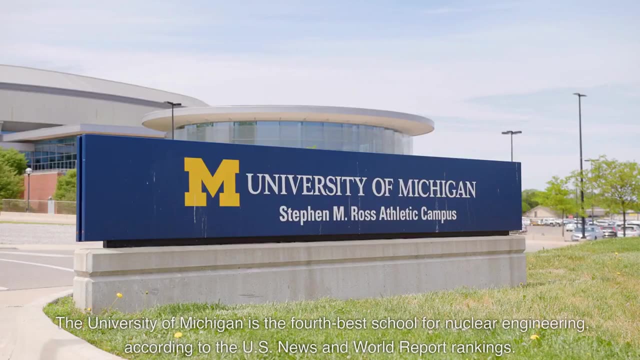 The University of California, Berkeley is another great option for aspiring nuclear engineers. It offers a wide range of courses in the field, including advanced topics such as heat transfer, fuel cycle technologies and radiation shielding. 4. University of Michigan: The University of Michigan is the fourth-best school for. 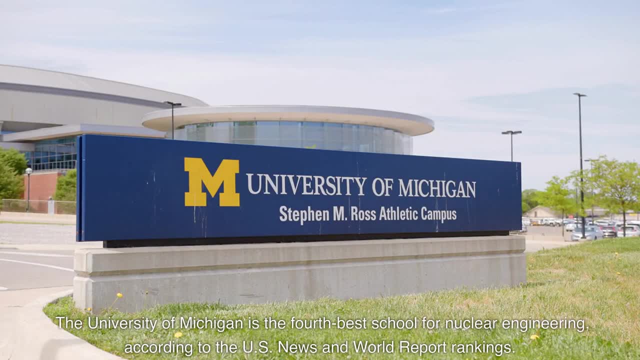 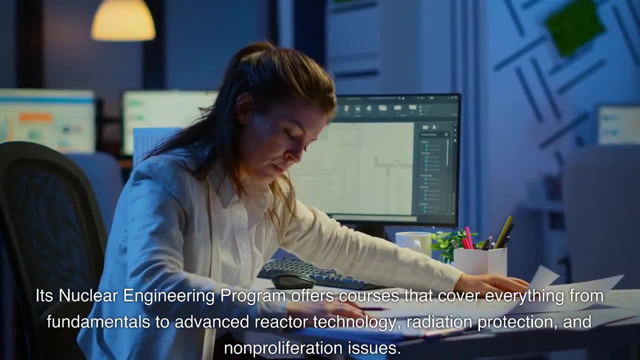 nuclear engineering in the world. It is the fourth-best university in the world for nuclear engineering According to the US News and World Report rankings. Its nuclear engineering program offers courses that cover everything from fundamentals to advanced reactor technology, radiation protection and nonproliferation issues. 5. University of Tokyo. 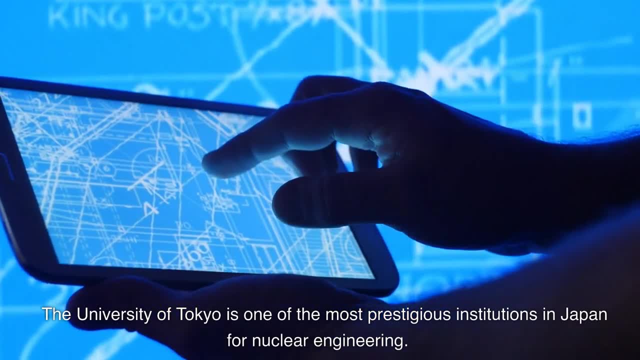 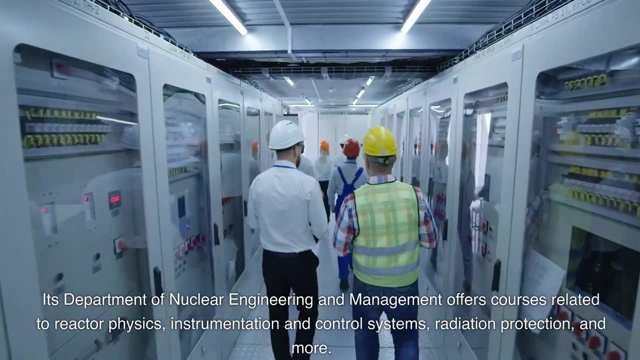 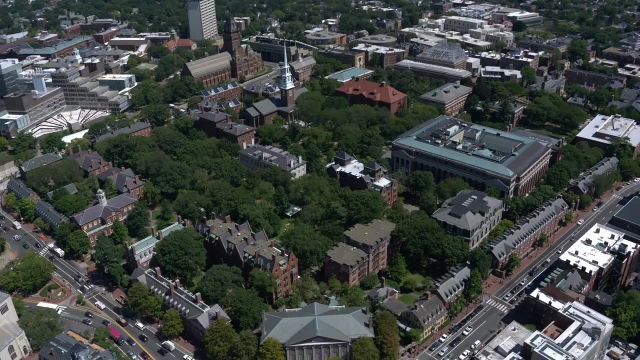 The University of Tokyo is one of the most prestigious institutions in Japan for nuclear engineering. Its Department of Nuclear Engineering and Management offers courses related to reactor physics, instrumentation and control systems, radiation protection and nuclear engineering. 6. University of Cambridge: The University of Cambridge is another great 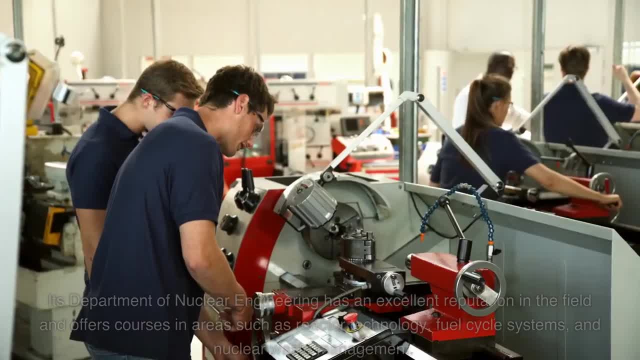 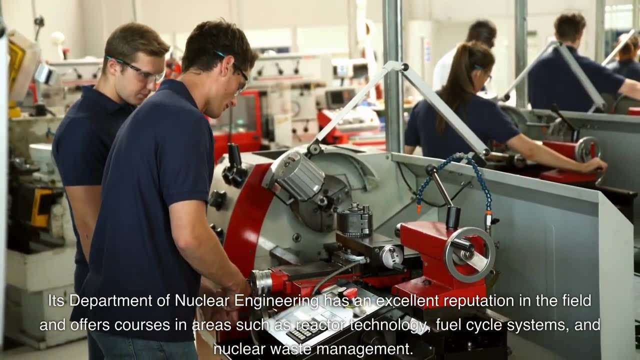 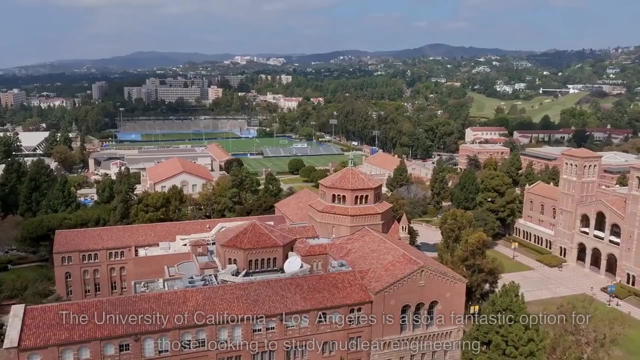 choice for those considering a career in nuclear engineering. Its Department of Nuclear Engineering has an excellent reputation in the field and offers courses in areas such as reactor technology, fuel cycle systems and nuclear waste management. 7. University of California, Los Angeles. The University of California Los Angeles is also a fantastic option for those looking to study nuclear engineering. 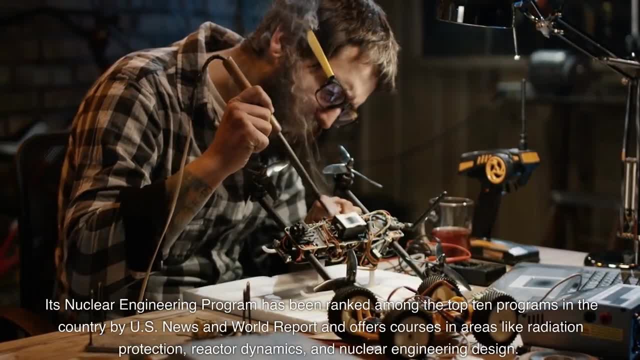 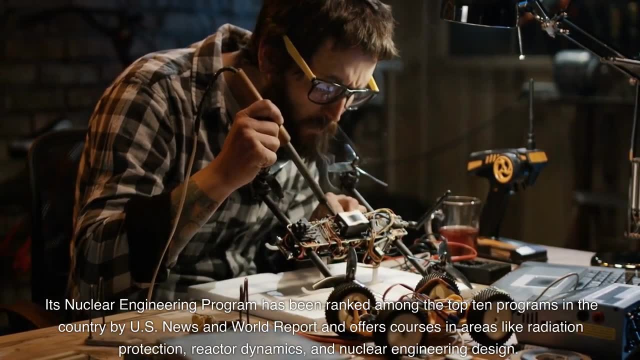 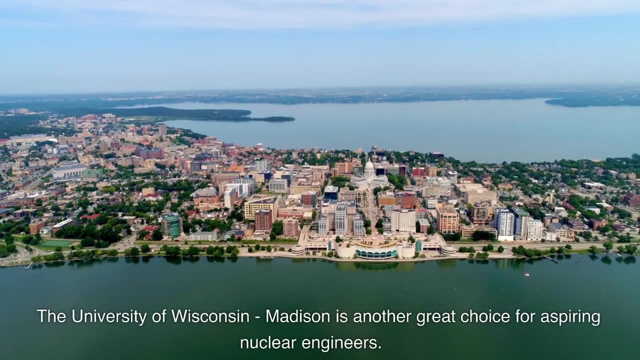 Also, its nuclear engineering program has been ranked among the top ten programs in the country by US News and World Report and offers courses in areas like radiation protection, reactor dynamics and nuclear engineering design. 8. University of Wisconsin Madison. The University of Wisconsin Madison is another great choice for aspiring nuclear engineers. 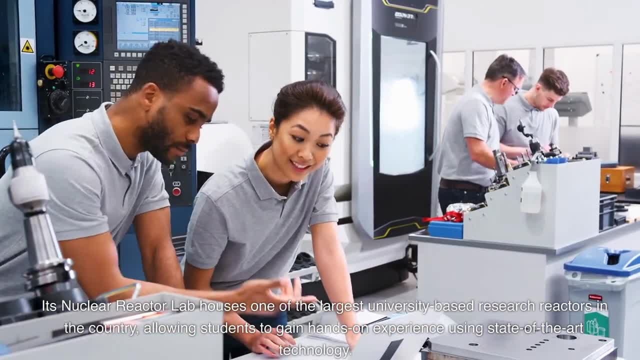 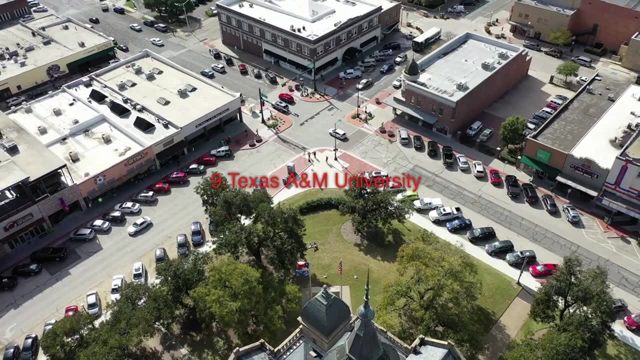 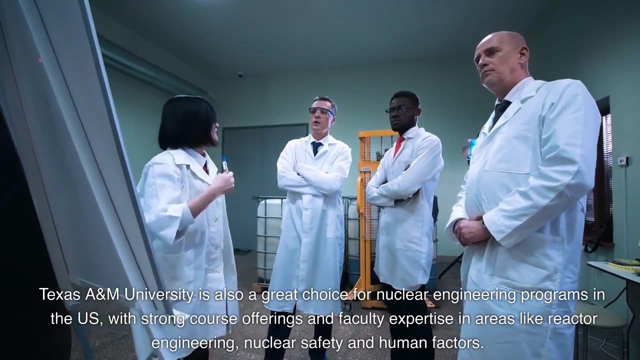 Its nuclear reactor lab houses one of the largest university-based research reactors in the country, allowing students to gain hands-on experience in the field of nuclear engineering- experience using state-of-the-art technology. 9. Texas A&M University. Texas A&M University is also a great choice for nuclear engineering programs in the US. 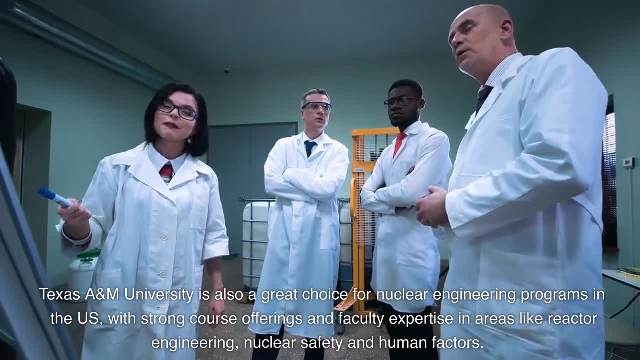 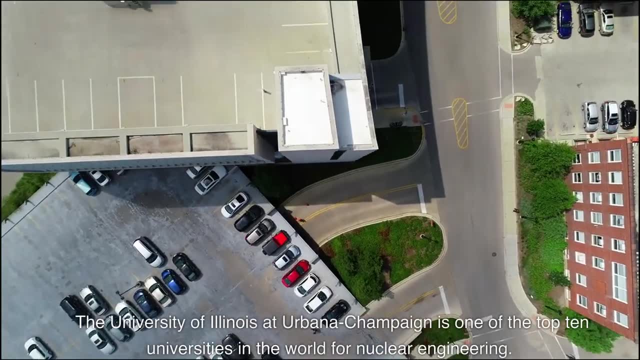 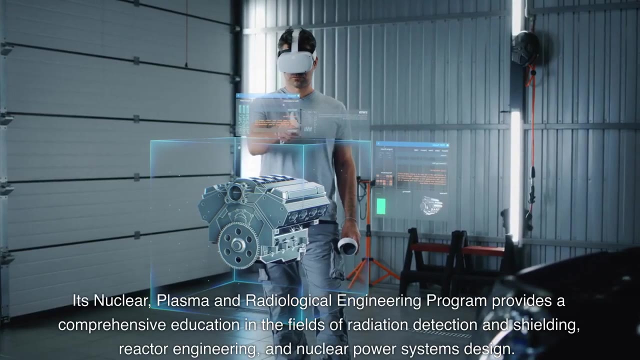 with strong course offerings and faculty expertise in areas like reactor engineering, nuclear safety and human factors. 10. The University of Illinois. The University of Illinois at Urbana-Champaign is one of the top 10 universities in the world for nuclear engineering. Its Nuclear Plasma and Radiological Engineering Program provides. 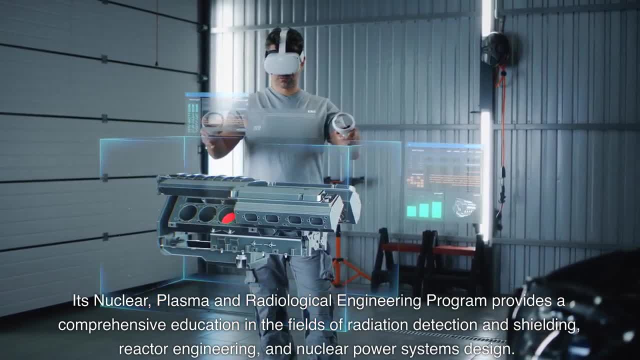 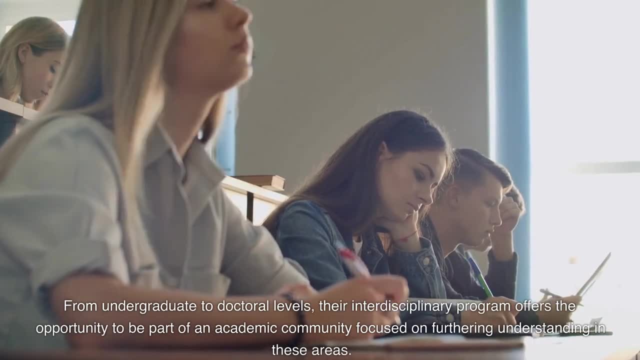 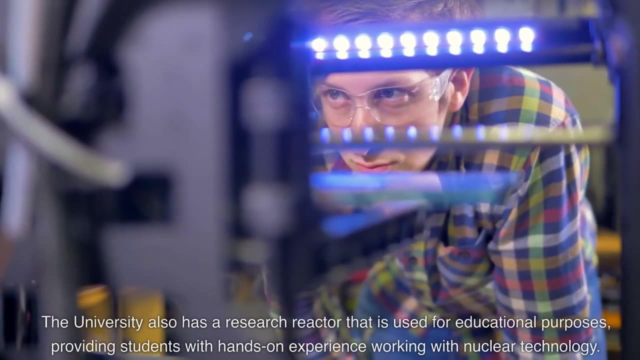 a comprehensive education in the fields of radiation detection and shielding, reactor engineering and nuclear power systems design, From undergraduate to doctoral levels. their interdisciplinary program offers the opportunity to be part of an academic community focused on furthering understanding in these areas. The university also has a research reactor. 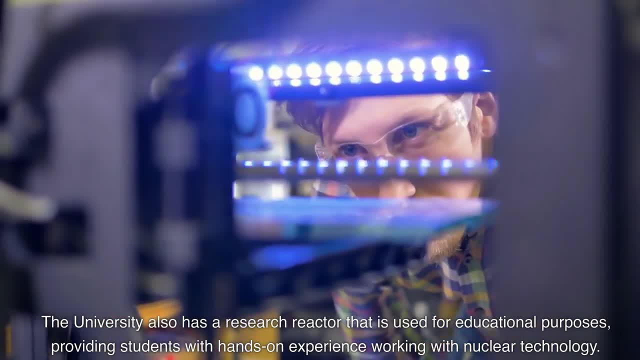 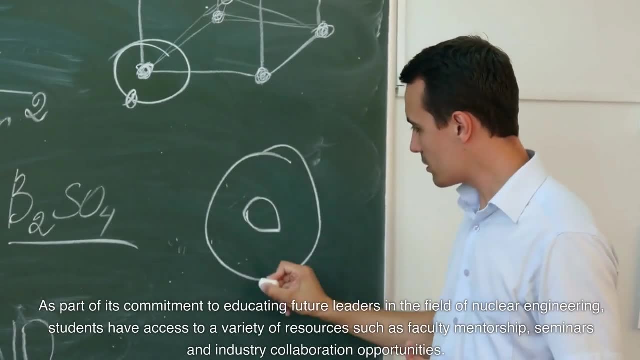 that is used for educational purposes, providing students with hands-on experience working with nuclear technology. 10. Texas A&M University. Texas A&M University is also a great choice for nuclear engineering- It's nuclear plasma and technology- As part of its commitment to educating future leaders in the field of nuclear engineering. 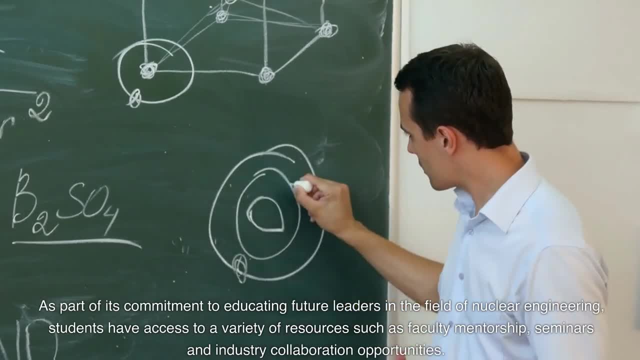 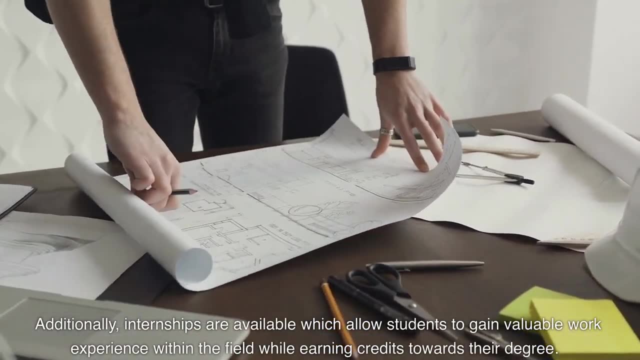 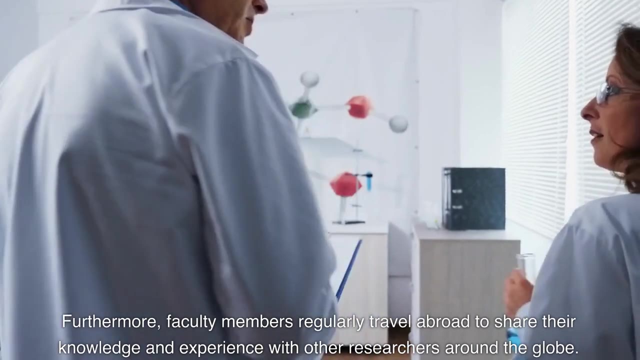 students have access to a variety of resources, such as faculty mentorship seminars and industry collaboration opportunities. Additionally, internships are available, which allows students to gain valuable work experience within the field while earning credits towards their degree. Furthermore, faculty members regularly travel abroad to share their knowledge. 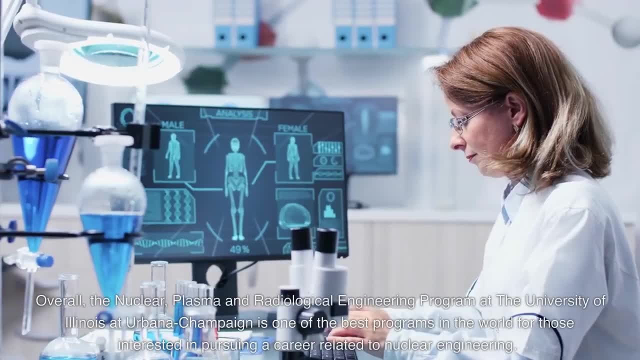 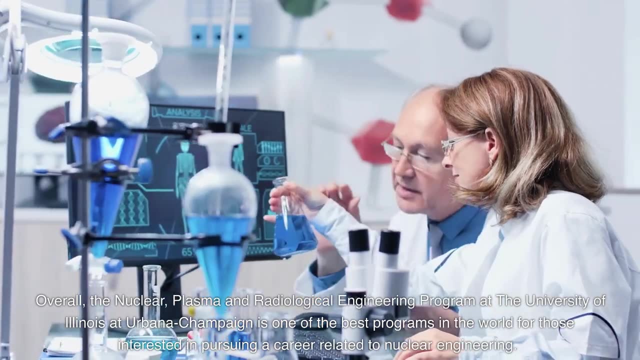 and experience with other researchers around the globe. Overall, the Nuclear Plasma and Radiological Engineering program at the University of Illinois at Urbana-Champaign is one of the best programs in the world for those interested in pursuing a career related to nuclear engineering.